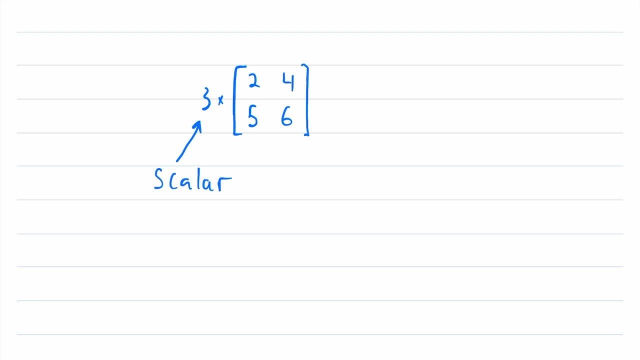 by itself is called a scalar, And that, of course, is why this is called scalar multiplication. we're multiplying a scalar by this matrix, So what do you think is going to happen here when we multiply this matrix by a scalar of three? you might think that the most natural way to 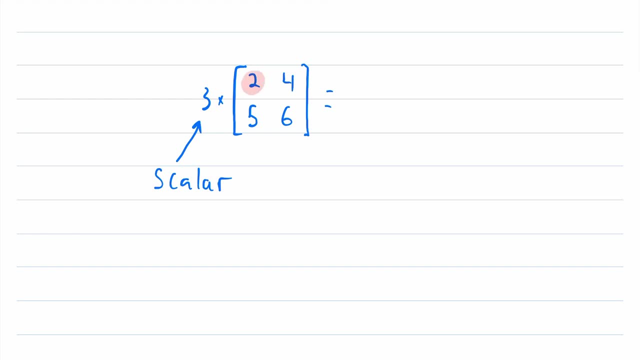 define this operation would be to multiply each of these matrices by a scalar of three. So what do you think is going to happen here when we multiply this matrix by a scalar of three? you might think that the most natural way to define this operation would be to multiply each entry in. 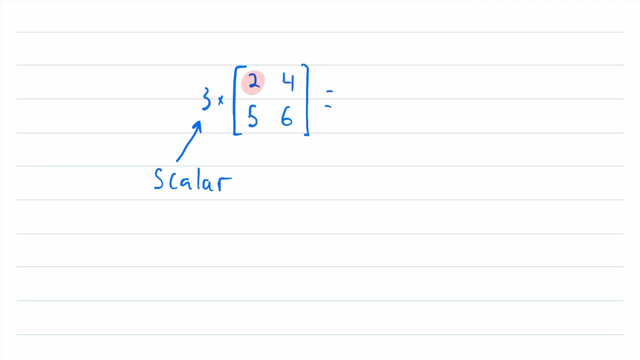 the matrix by the scalar, And you would be right. that is how we define scalar multiplication. So three multiplied by this matrix gives us another matrix with the exact same dimensions And the entries are two actually. I'll write it like this: three times two, and then three times four. 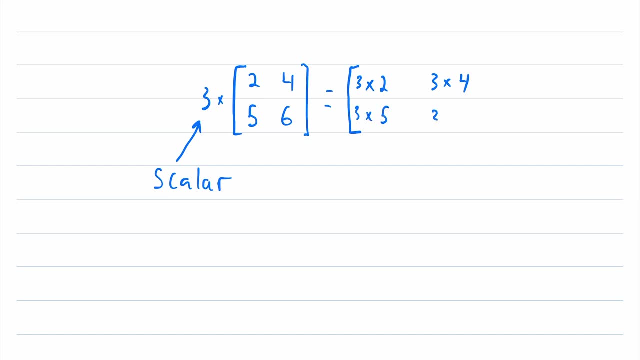 and then three times five and then three times six. So when we multiply a matrix by a scalar, we get a matrix with the exact same dimensions, just multiplying each entry by the scalar. So, finishing this up, let me move this to the left And we'll write what this matrix is equal to: three. 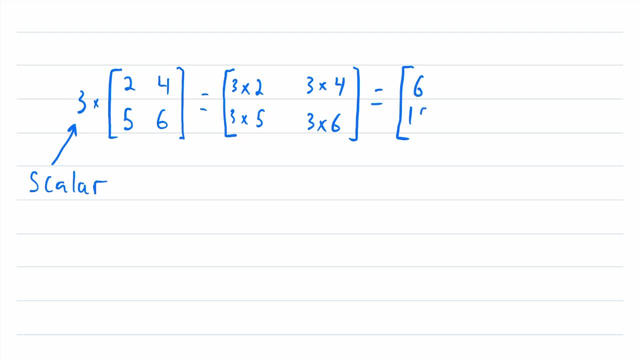 times two is six, three times five is 15.. Three times four is 12. And three times six is 18.. So, when we multiply a matrix by a real number, that is called scalar multiplication, And that's what we're going to do, And to carry out this operation, all we have to do is multiply each. 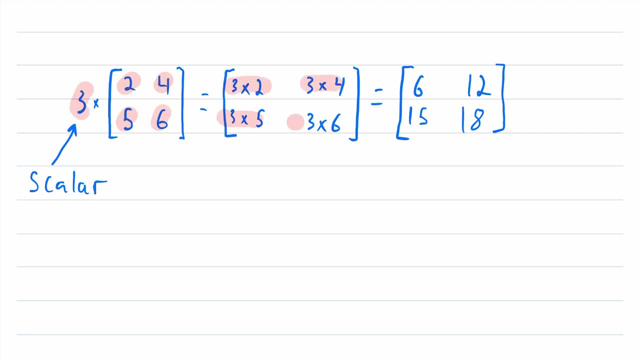 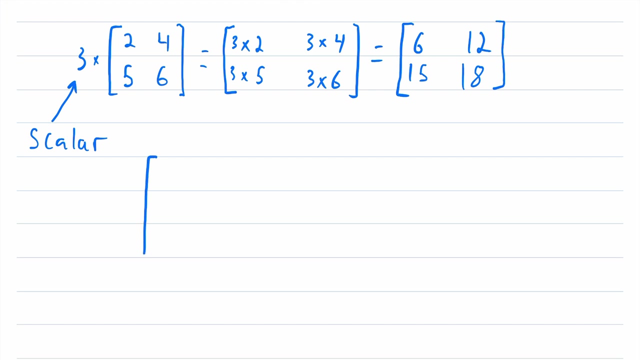 entry of the matrix by the scalar. I think it's pretty intuitive And I'll also point out that the order does not matter. it's pretty natural to put the scalar before the matrix, But you could also put the scalar after the matrix. For example, let's say we had this: three by one matrix entries. 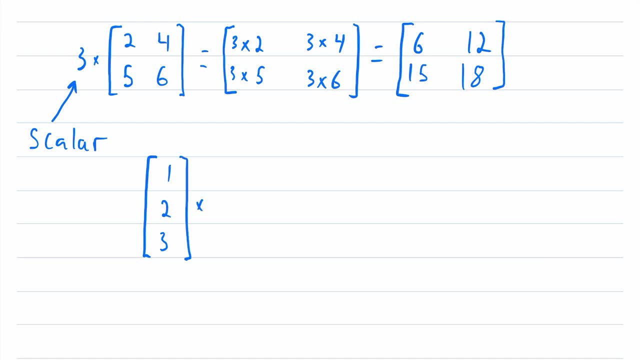 one, two, three, and we could multiply it by a scalar of negative three times four, And we could multiply it by a scalar of negative three times four, And we could multiply it by a scalar of negative two, And this would work just the same way. we multiply each entry in the matrix by the. 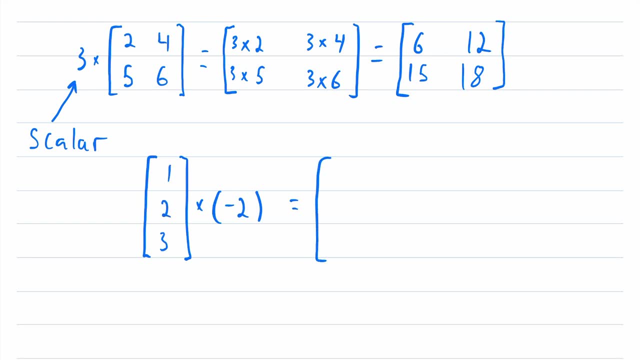 scalar of negative two. So this is going to give us one times negative two, which will be negative two, two times negative two, which will be negative four, and three times negative two, which will be negative six. So when we're dealing with real numbers, scalar multiplication is commutative.